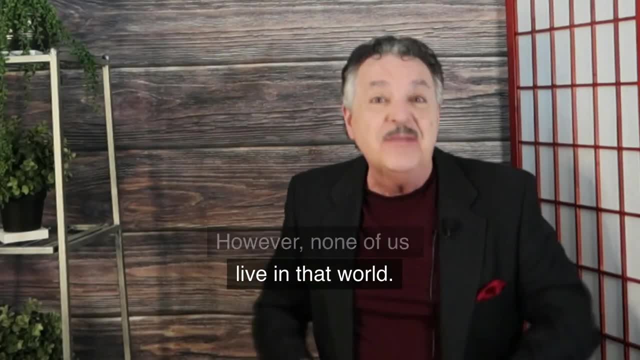 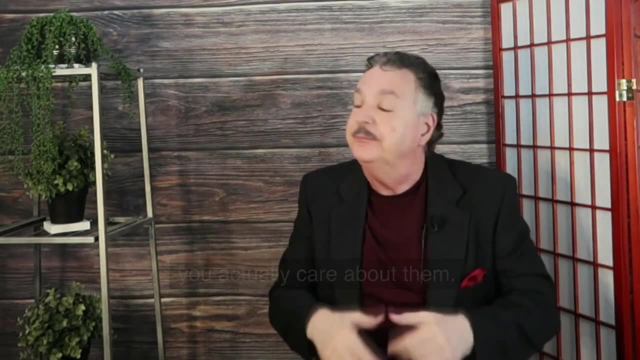 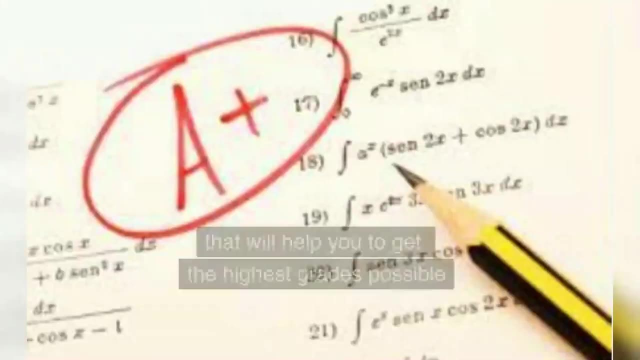 they were being tested on. However, none of us live in that world. Often there are classes you're required to take whether or not you actually care about them. I'm not here to debate that. My goal is to show you simple, proven strategies that'll help you to get the highest. 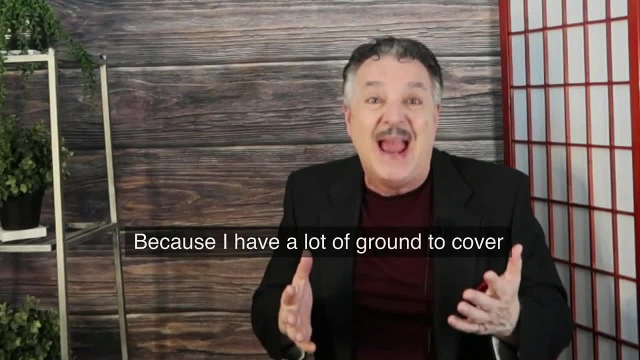 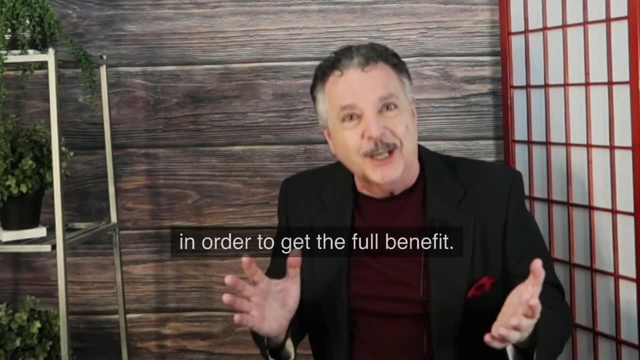 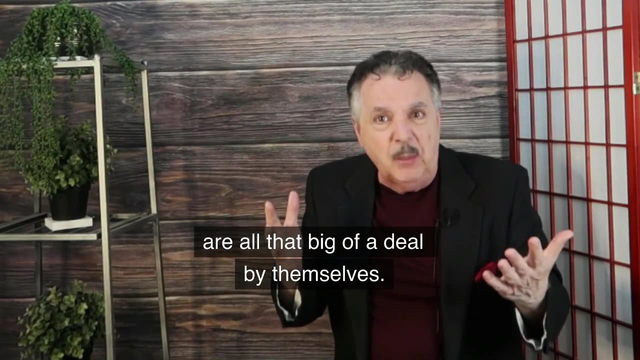 grades possible on multiple choice tests Out of ground to cover. this is part one of a two-part series. Be sure you also watch part two in order to get the full benefit. Also, be warned in advance. None of the strategies you're going to get are all that big of a deal by themselves, In fact you may think. 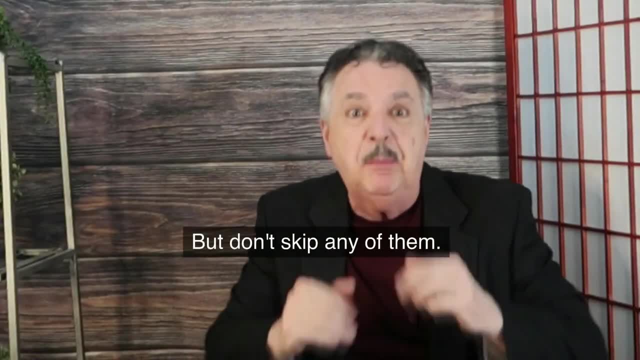 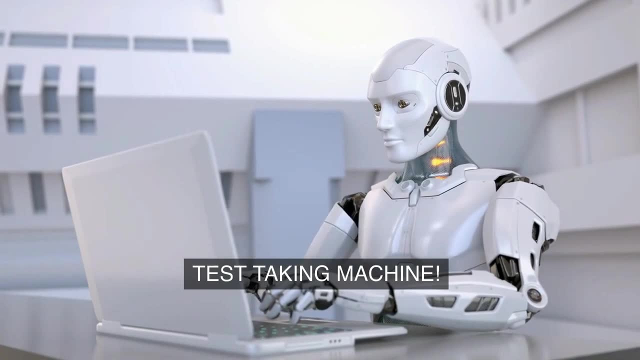 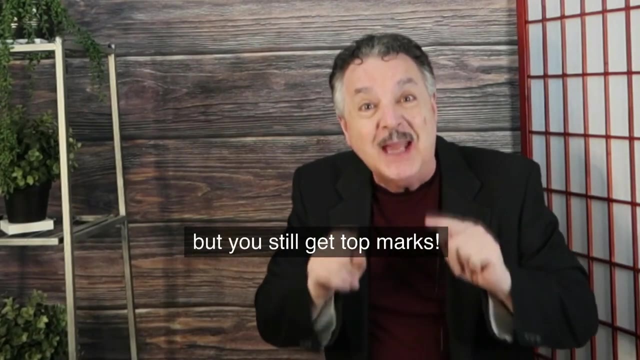 of some of them as simply common sense, but don't skip any of them. You see, when you combine the strategies together, you can become a test-taking machine. Others will envy you because you don't seem to work that hard, but you still get top marks. 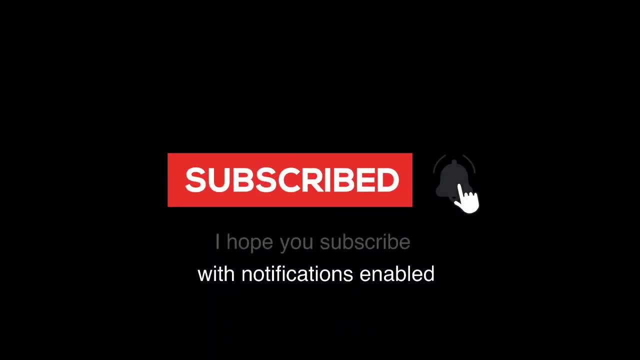 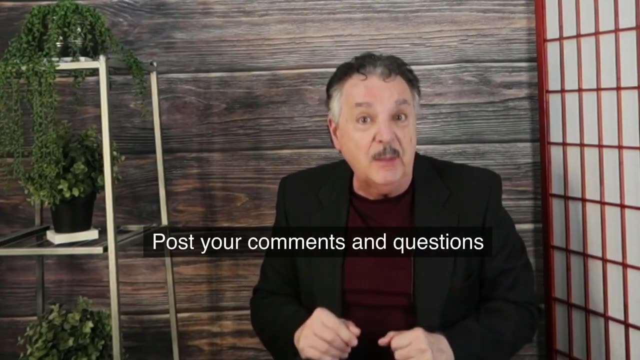 If you haven't done so yet, I hope you subscribe with notifications enabled with that little bell icon, so you'll always know when I release a new video. Post your comments and questions, because I pay attention to them, And so does YouTube. 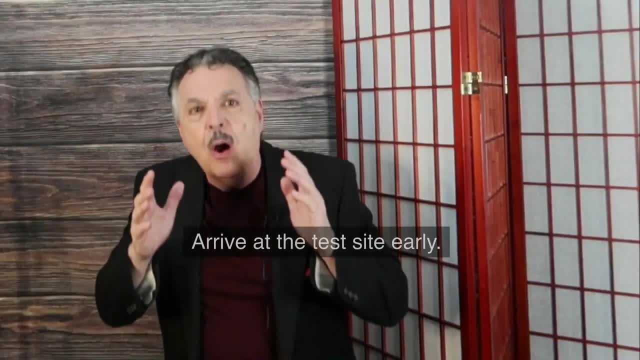 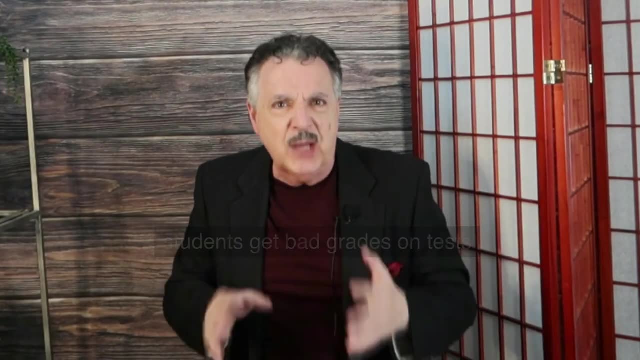 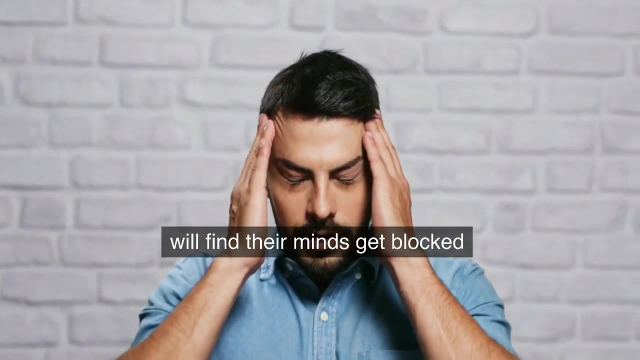 Okay, let's get started. Tip number one: Arrive at the test site early. The single biggest reason Students get bad grades on tests has more to do with stress than anything else. Even students who know the answers will find their minds get blocked when they're feeling too. 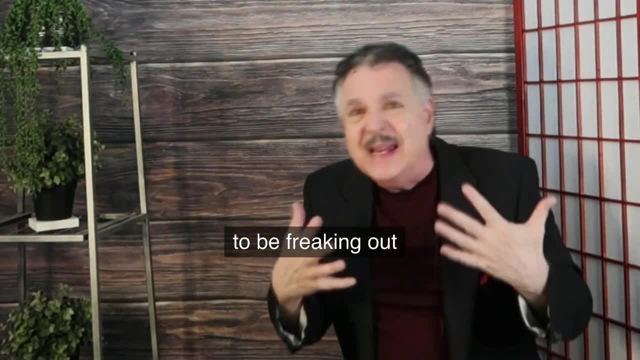 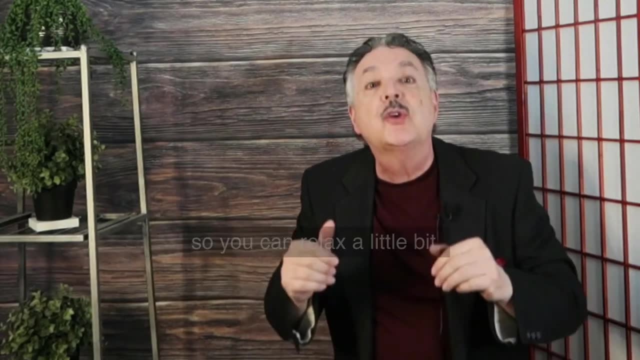 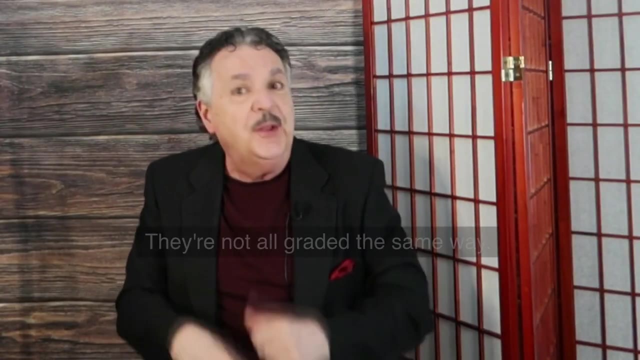 much stress. The last thing you want is to be freaking out because you're hoping to get to the test on time. Get there with plenty of time to spare so you can relax a little bit. Number two: Know how the test will be scored. They're not all graded the same way. They all have different answers. Do you get penalized more for a wrong answer compared to an answer you leave blank, Maybe, Or is it the other way around and you're penalized more for blank answers than wrong ones? Don't just assume they're graded the same way. 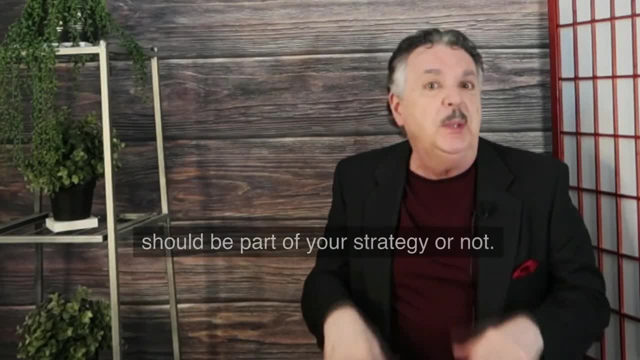 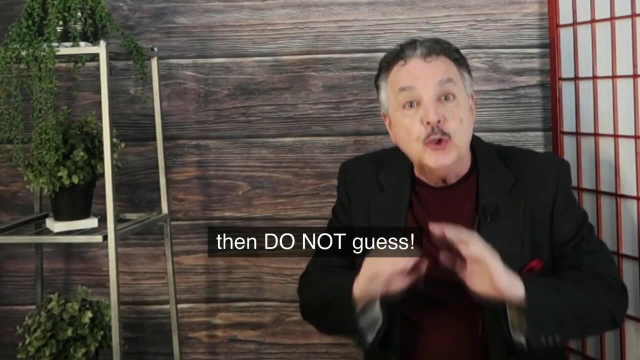 In other words, it's good to know whether guessing should be part of your strategy or not. If blank answers don't count as much against your grade, then do not guess. If you're graded the same for a blank answer as a wrong one, you're probably going to get. 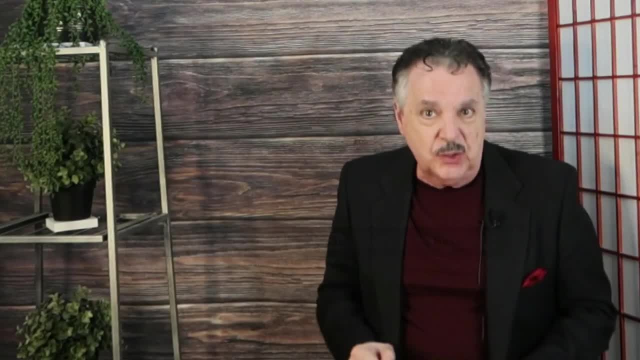 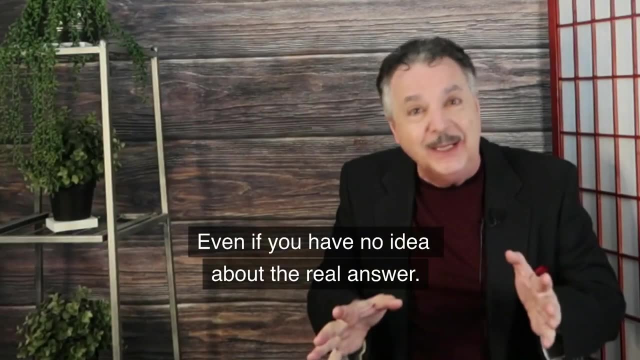 the wrong one, then you absolutely want to guess. If there are five possible answers, you have a 20% chance of getting it right, even if you have no idea about the real answer, And 20% is better than 0%. 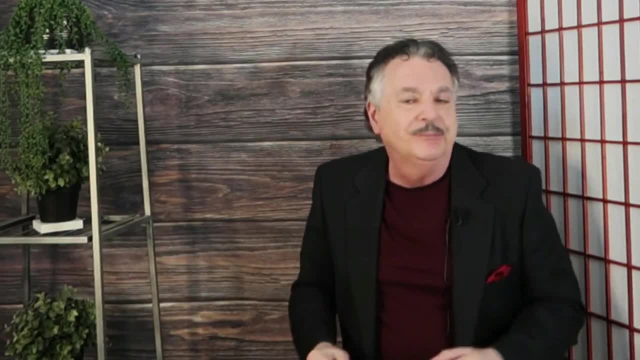 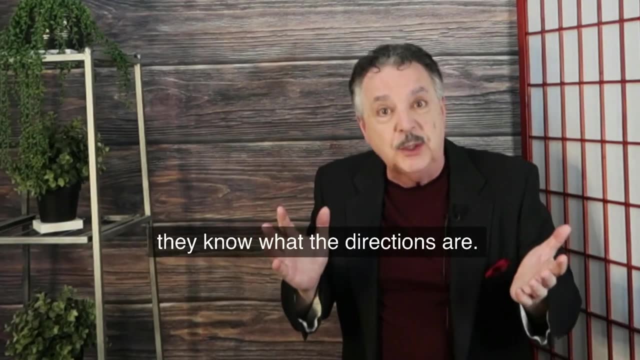 Number three: Read the directions carefully. I know that sounds like it should be obvious, but there are tons of students who simply assume they know what the directions are. For example, The directions might say something like: The directions might say something like: 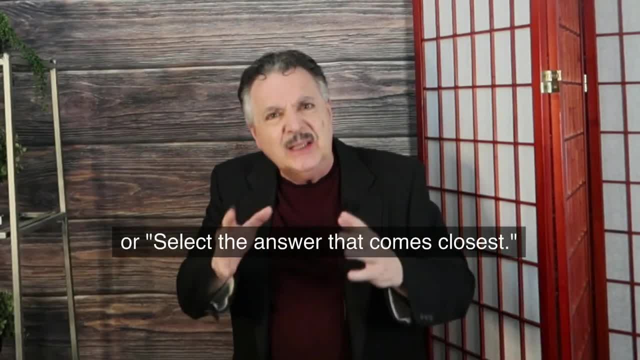 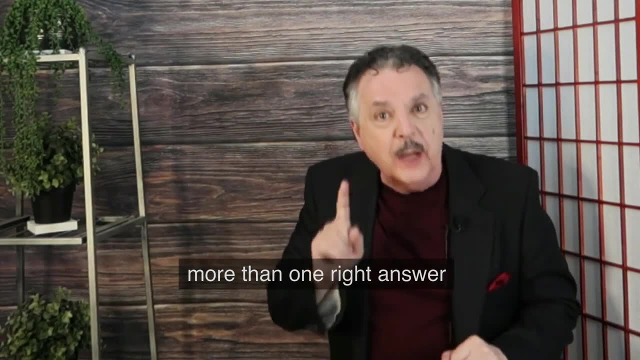 The directions might say something like Select the most correct answer Or select the answer that comes closest. Whenever you see something like that, you're being told that there may be more than one right answer Or shades of right or wrong within the answers. 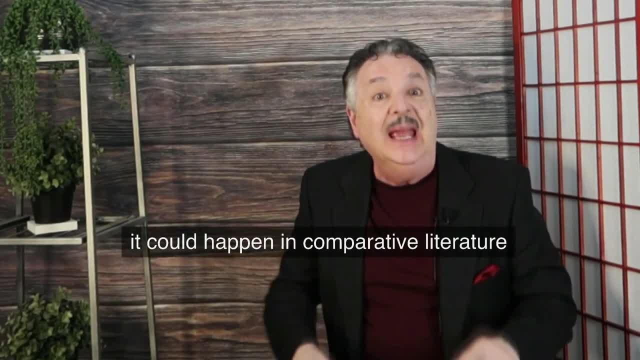 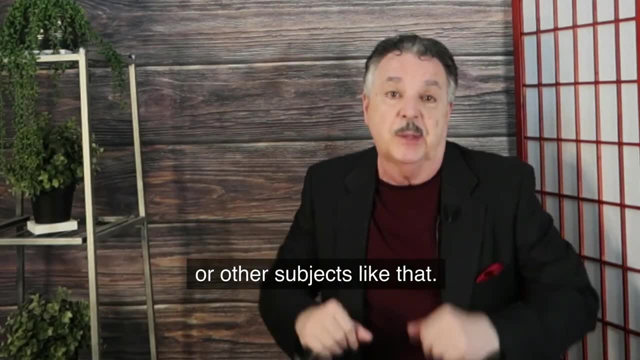 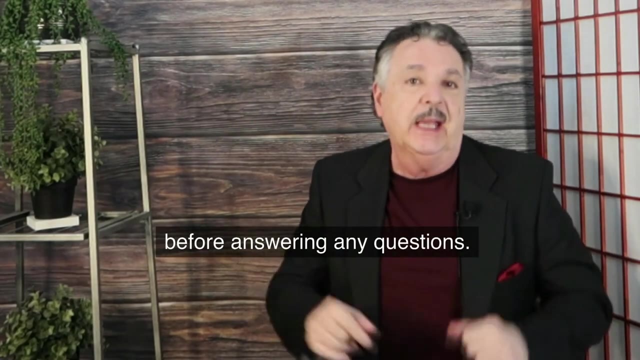 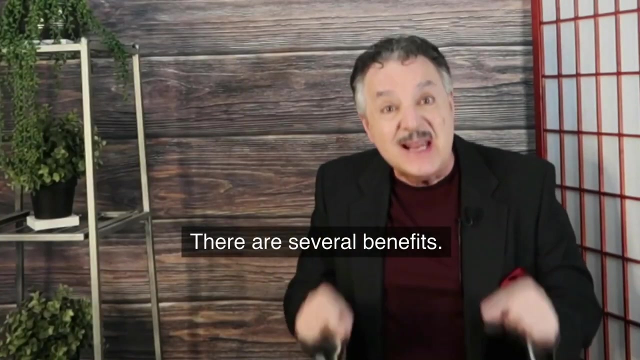 While that may not happen in science or math tests, it could happen in comparative literature or psychology or sociology or other subjects like that. Number four, Number four: If possible, read the entire test before answering any questions. Of course you want to do it fast and not waste any time. there are several benefits. 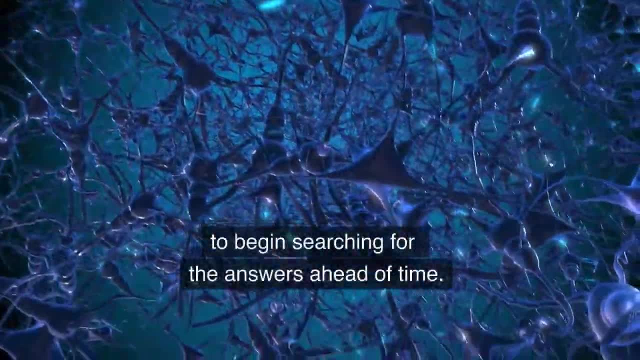 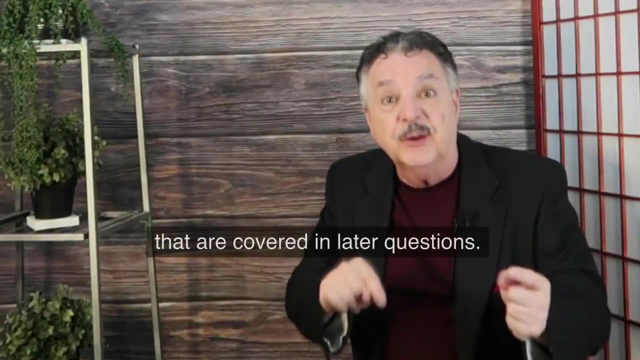 First, it prepares your subconscious mind to start searching for the answers ahead of time. Next, sometimes you'll get answer clues for early questions that are covered in later ones. Also, If you're well-prepared, it will give you a better feeling of confidence From time. to time you can get 8 or 9 correct answers in either question and it's almost jegis. you'll know what the whole test is about. Lastly, it helps you budget your time so you don't waste any on questions that are too hard when there are easier ones. 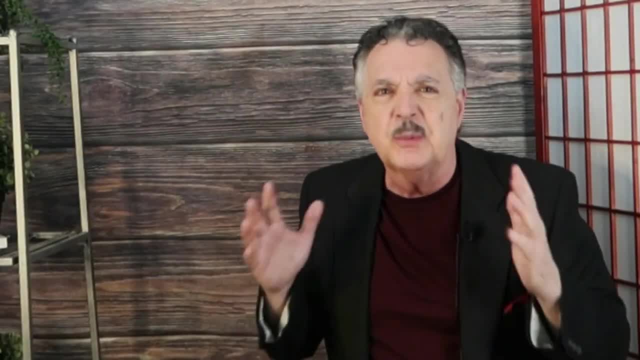 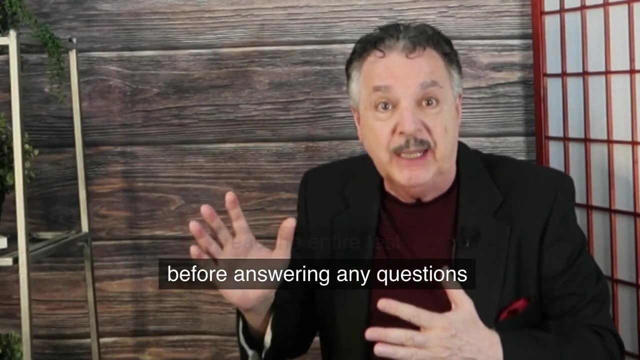 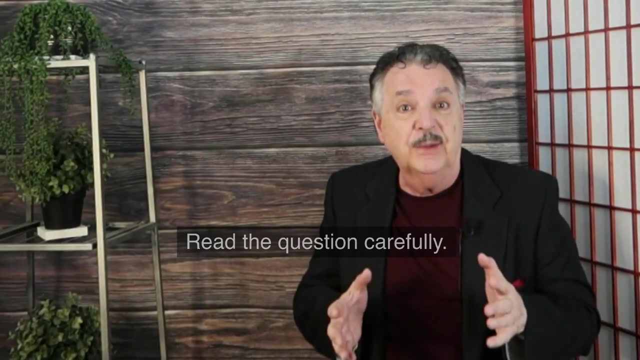 to answer first. I know this may not work with some standardized computer delivered exams, but remember, if it's possible, read the entire test before answering any questions and do it as quickly as you can. Number five: read the question carefully. Oof, this is a big one. Most mistakes are made because you. 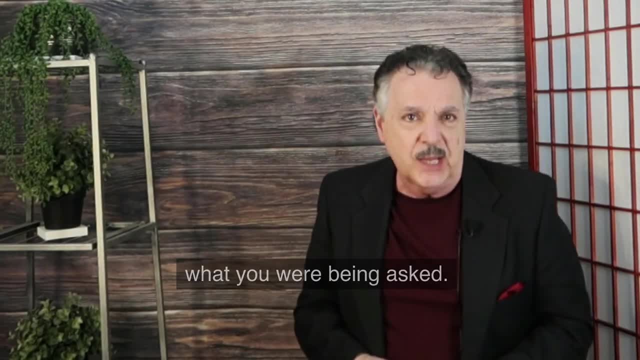 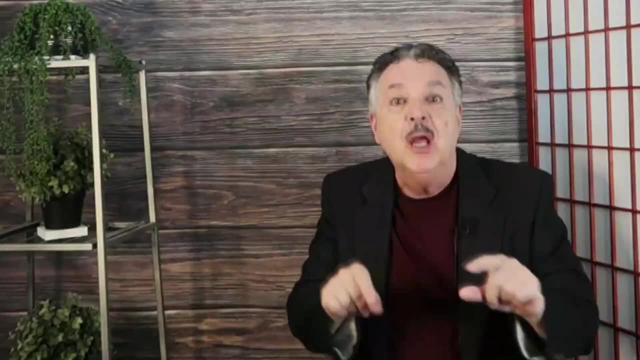 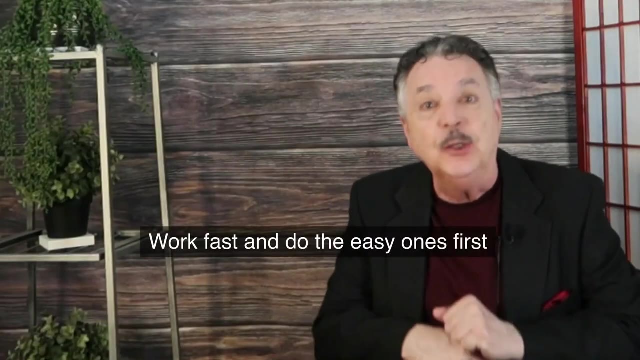 didn't clearly define what you were being asked. Don't jump to conclusions. read the entire question. target important keywords or phrases. Be sure you are answering what is being asked. Number six: work fast and do the easy ones first. Time management is a big part of being successful and taking tests.